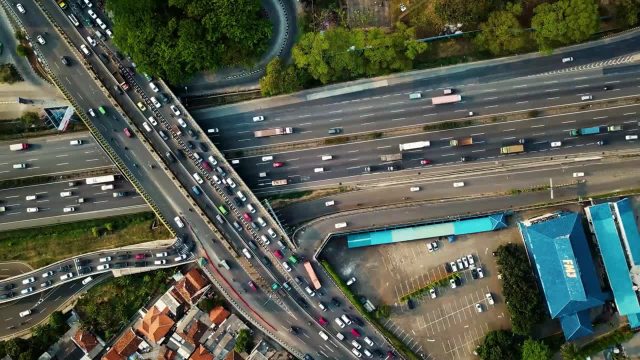 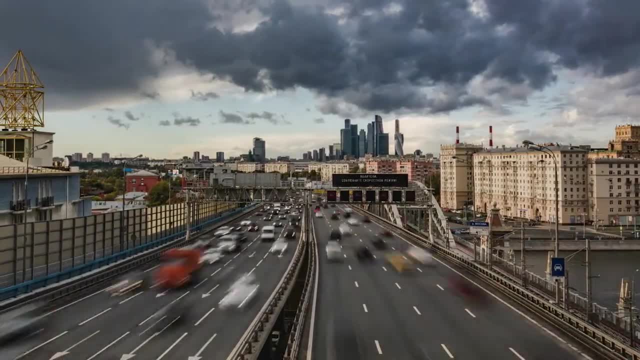 And long commute times, Which not only increases the frustration of residents living in the area, but it also increases the amount of fossil fuels being used and the amount of air pollution, Which increases the area's carbon footprint, Reducing the air quality for all residents. Living in the area And reducing the overall health of citizens. Speaking of pollution, we can see that heavily densely populated areas that lack sustainable measures often times lack public transportation, Which means more people will drive to work, to the grocery store or to get the goods and services they need. Which means more cars on the road, Which in a low densely populated area isn't the end of the world, But in a heavily densely populated area we see that more air pollution going out into the city, Which creates smog and lowers the overall quality. Which increases the overall quality of air for all residents. We can see similar things happening as well with the water supply, As more and more pollutants get into the local lakes and rivers and oceans. All of this decreases the standard of living and health for residents in the area. 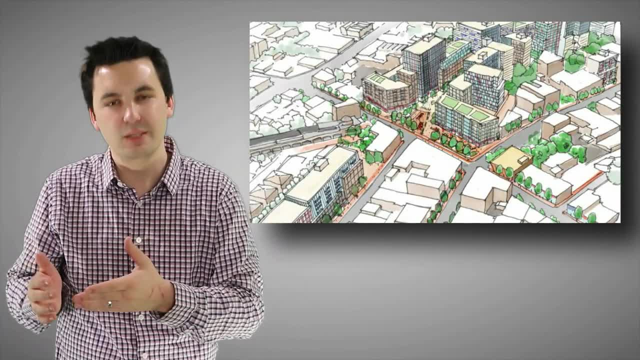 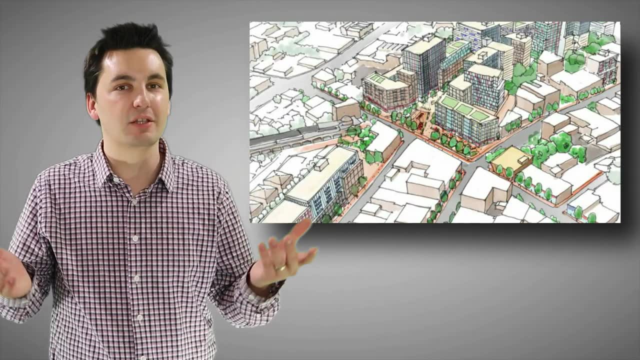 Using things like smart growth policies, new urbanism, green belts and also green energy Are great ways to try and increase the standard of living for people in a city And also make their cities more sustainable. Cities can also rezone and redevelop land. 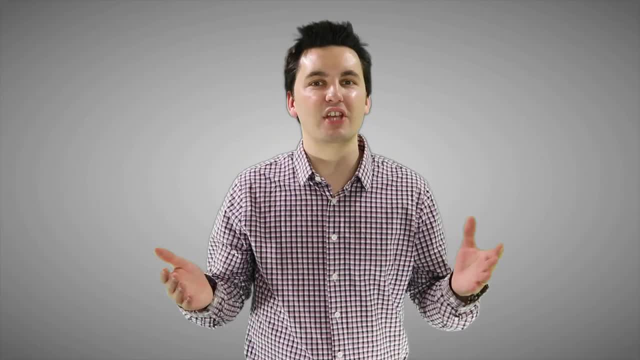 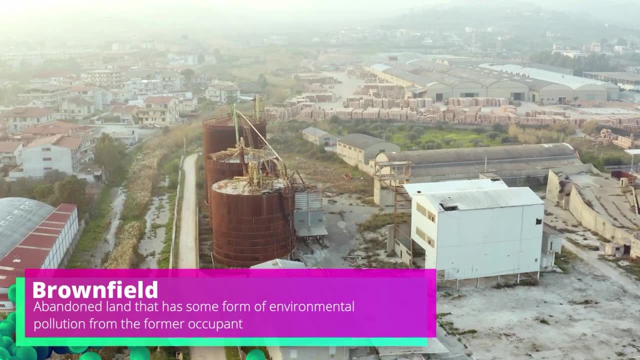 That has been polluted and is no longer being used. For example, we could look at brownfields, Which is land that's been abandoned and has been left polluted by the former occupants who used to reside there. Brownfields may have been used as industrial work, a former landfill or even a gas station. 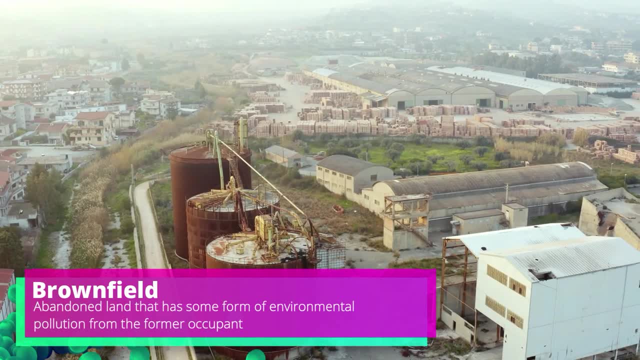 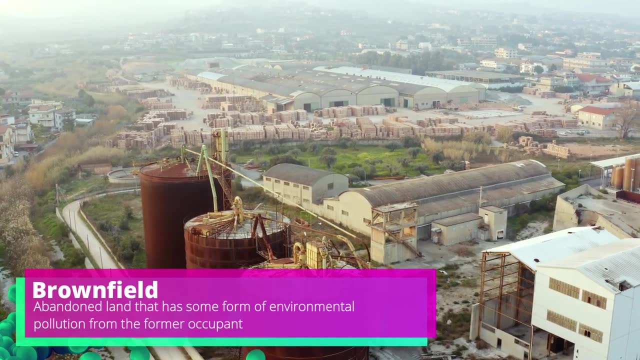 Typically, the former occupant left the land contaminated, Causing it to remain empty. Cities can work to redevelop this contaminated land And rezone it to create new communities in it And better utilize their land space, And all the while creating a more sustainable city. 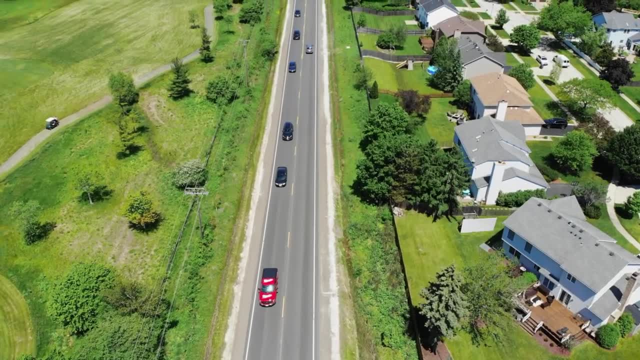 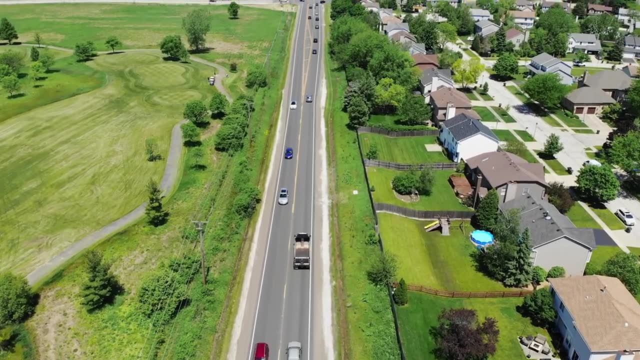 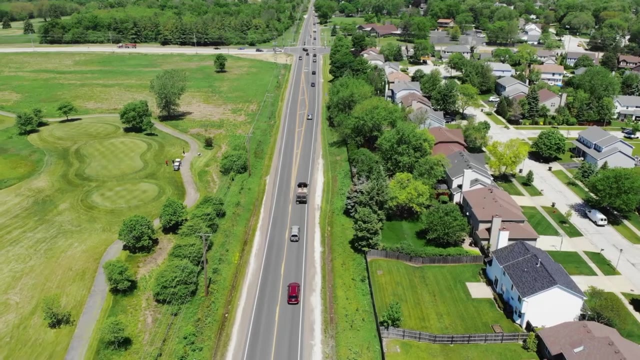 Lastly, we could also see cities promote urban sustainability By using farmland protection policies Which set restrictions on development to prevent further destruction of farmlands, Or cities that implement urban growth boundaries To prevent the further expansion of a city through urban sprawl. 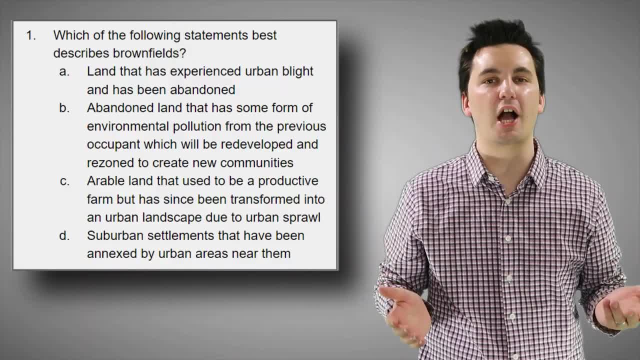 And just like that, geographers, we're done with another unit of AP Human Geography. It's kind of funny. it seems like just yesterday we were starting unit 1. And now we're on to unit 7. And we're almost done with the course. 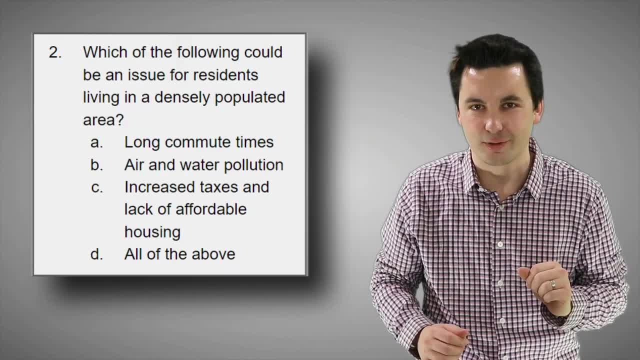 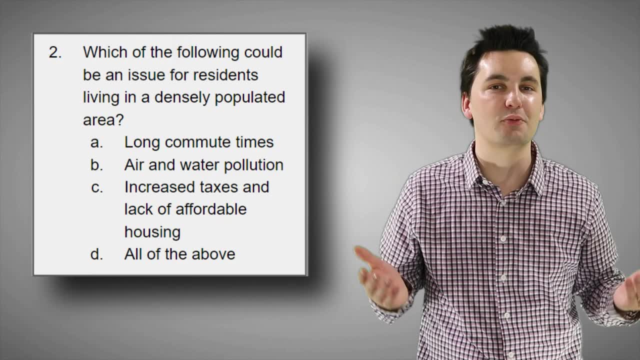 But before we get too ahead of ourselves, Make sure you answer the questions on the screen right now And check your answers in the comments below While you're down there. of course, too, Consider subscribing and liking the video- Great way to say thank you for the videos. 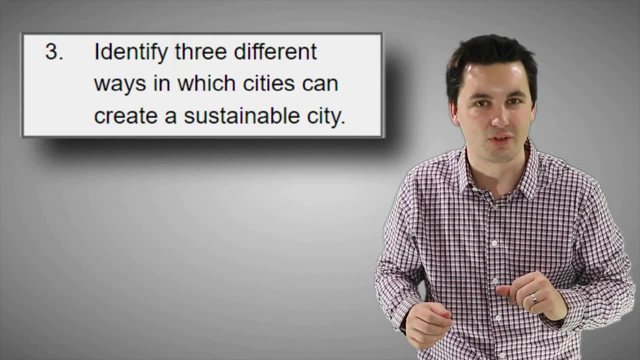 And make sure that I can make more videos in the future. And make sure you don't miss the unit 7 videos Plus, don't forget to check out that unit 6 summary video. It'll help you in your class and also on the national exam.